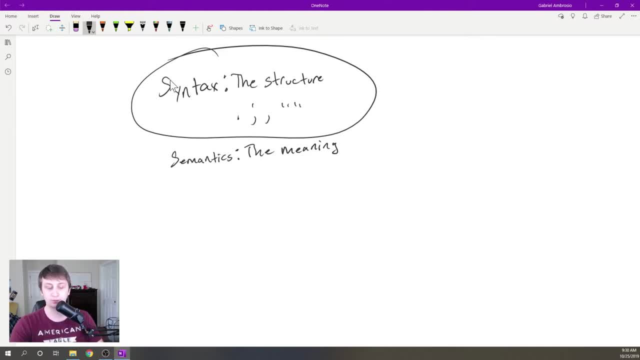 is correct. And so how does this translate to programming? So we know that the syntax is the structure of a natural language. We know the semantics is the meaning. Well, in programming it's the same thing. So the semantics in a programming language are just. 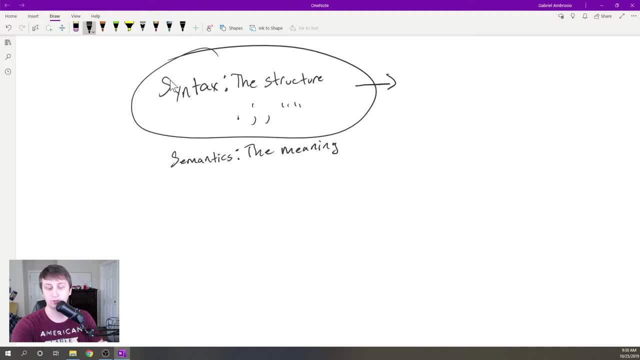 things like making sure that you're using proper variable names. So if you make a variable all lowercase V-A-R, you can't try and reference it by saying V, capital A-R. That's bad syntax And the programming languages are very strict on this. If you have anything wrong with your syntax, 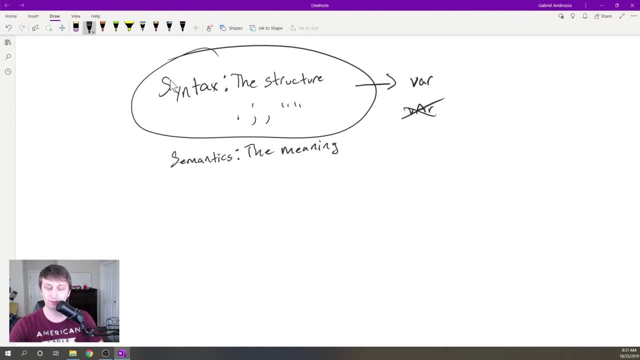 it's going to throw an error and it's going to tell you to fix that. Okay, And so other things that are syntactical with programming language are things like uh, semicolons as well um, keywords. So in Python that would be something like um. 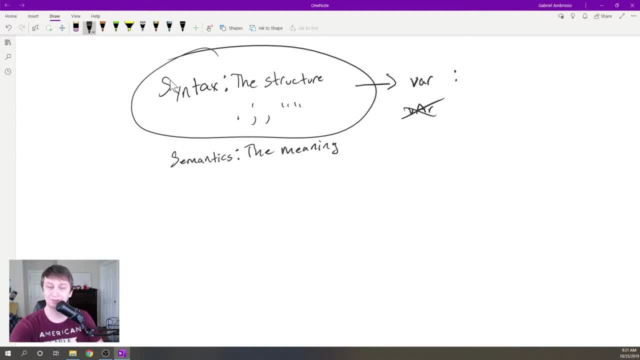 if string. uh, these are things we'll get to in the future. I don't want to go to into too too much depth, but as we hit those, I'll highlight. this is a keyword. Uh, this is important because this is part of the syntactical structure of the language. 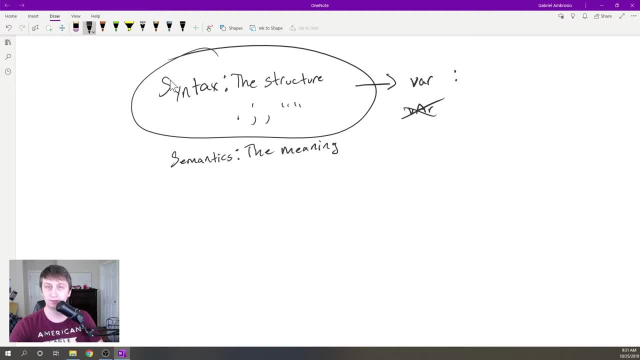 Okay, And then other parts of syntax of the language are just things like tabs in Python. If you have something indented one space, then everything must be indented that same space, or otherwise it will not work. So if you have some variable here, 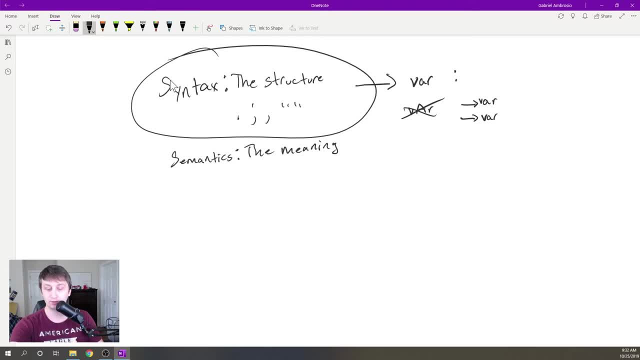 then the next variable. here these are all considered the same block, And we'll get into that a little bit more too, but I basically just want to convey: make sure that when I'm typing something on the screen, you are typing it exactly. 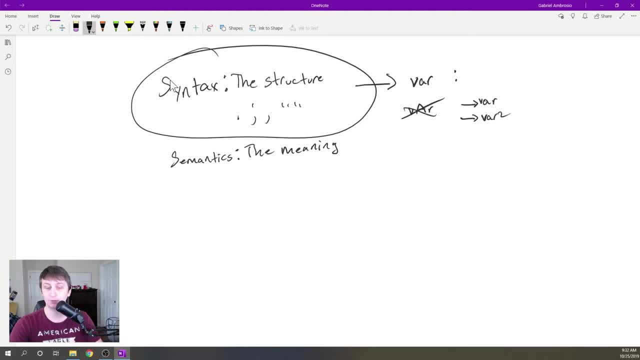 the same way, because otherwise it will not work, because the programming languages are very strict. They do give you some malleability with the way you form your meaning, but you have to follow the syntax pretty strictly. And so then, what is the semantics, the meaning of the programming language? 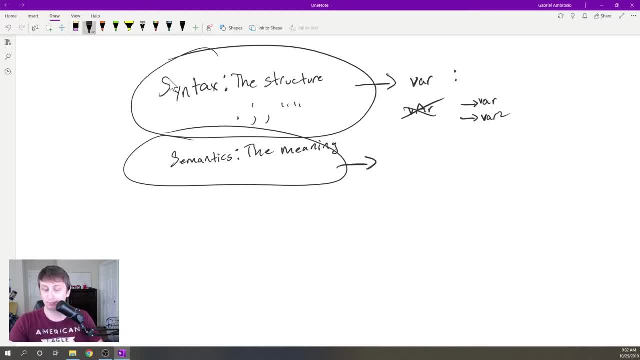 Well, if we translate this over to a programming language, this would just be different ways to say the same thing, And so, like I said, in English you have two different ways that you can say the same sentence and convey the same meaning. 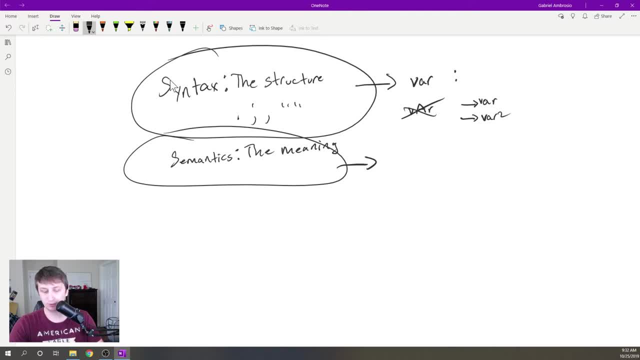 Likewise in programming. there are several ways to do one thing. You can declare a variable several different ways, and then you can also solve problems several different ways. It's sort of like mathematics too. So if I gave you a problem that said x equals 5 plus y and I said to solve for y, well, 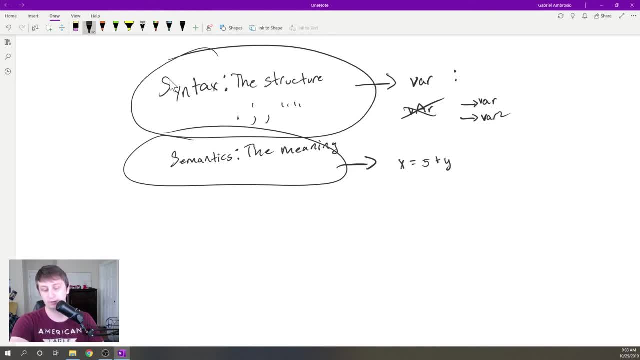 you could do two things. You could say: let's subtract y over, and then this would be: minus y plus x equals 5. Subtract x over minus y equals 5 minus x, and then divide everything by negative: 1. y equals x minus 5.. 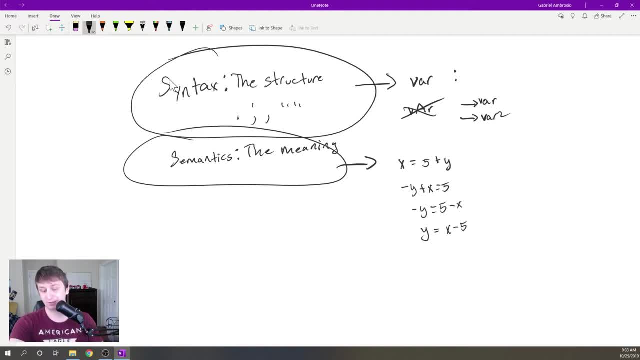 That's probably not the best way to do this. The other way to do this is much simpler. You just say: oh well, you could subtract 5 over y equals x minus 5.. And so this is something that's also important in programming languages, because you'll have: 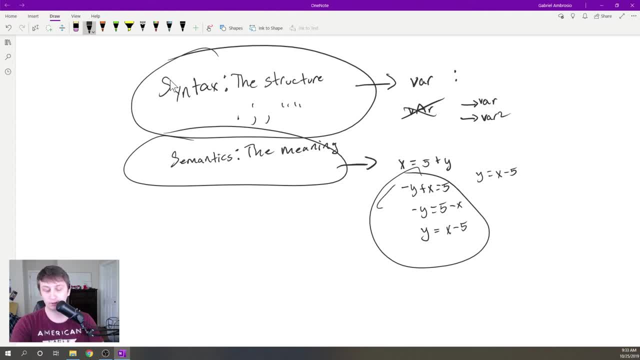 things like this where you can solve it this way. It's going to require a lot more steps and there might be a better way where you can solve it, But typically when you're programming something, I always go for solving it the most simple. 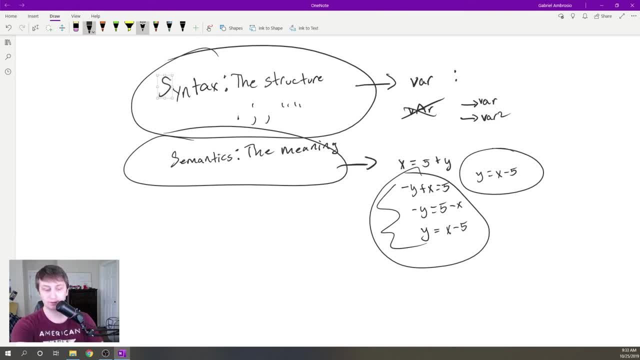 way, just finding something that works. This method works, so that's good. You could turn that in as a programming assignment and say, OK, this is my assignment, This is complete And that's fine. You solved it, That's good. 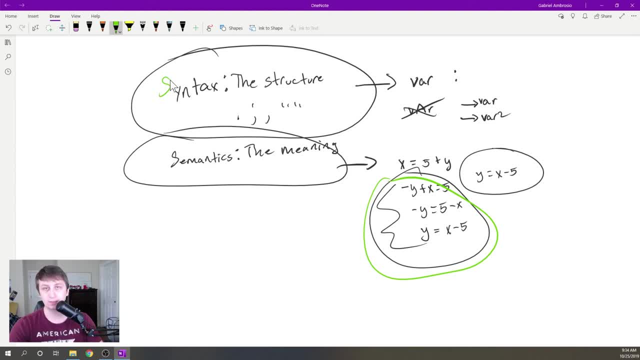 Then if it's causing difficulties with speed or anything like that, that's when you want to try and optimize and find a better solution, because then you might not have the best solution, You might not have the most optimal solution. There might not be a more optimal solution too. 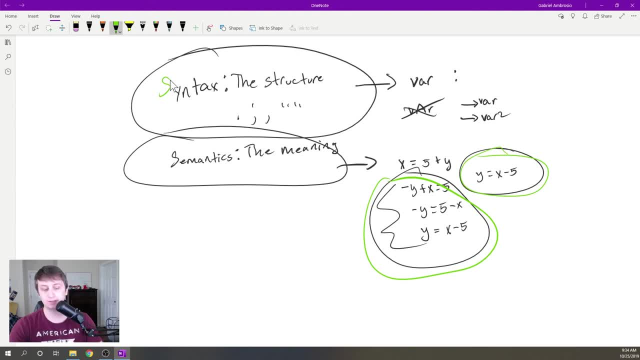 This might be the best that you can get to. So these are just two big things in programming- the syntax and the semantics- And I just want you to be aware: when I'm typing stuff, follow it exactly, Otherwise it will throw an error and it will say that that's not correct. 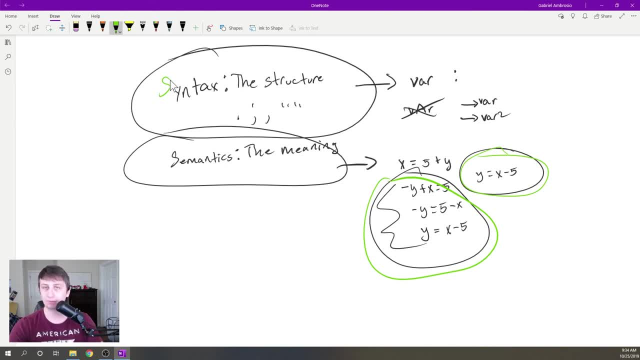 And then also just remember that when I'm solving something a specific way, that doesn't mean that's the only way to solve it. There's several different ways to solve programming problems, And I think there's a lot of creativity in that. 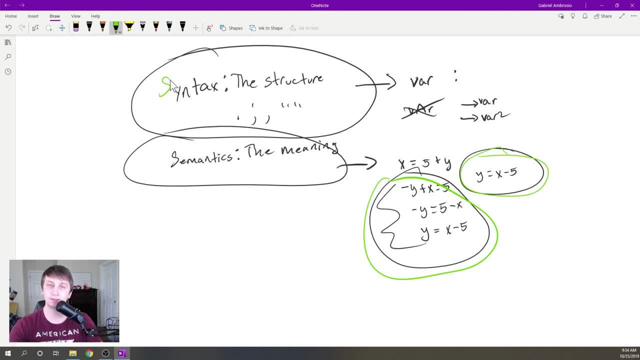 And that's something that we often- We often forget in mathematics and programming, since they're logical and concise professions. But there is a lot of different ways to do these things, And I encourage you to try several different ways to do the same thing, just that you learn.